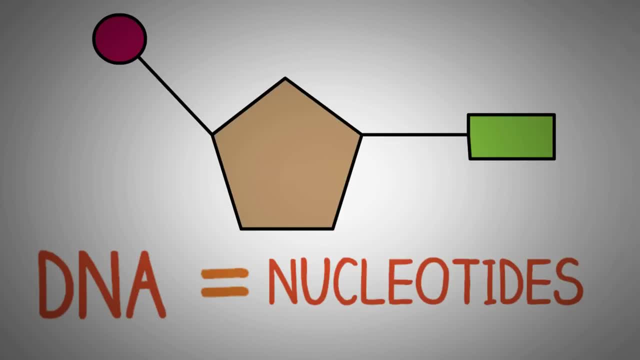 This is the basic structure of a nucleotide. You can see that it consists of three important groups: the phosphate, the sugar and the nitrogenous base. If you want to study the details of the structure of nucleotides, you can refer to the video about the nucleic acids. The link to that video will be in the description. 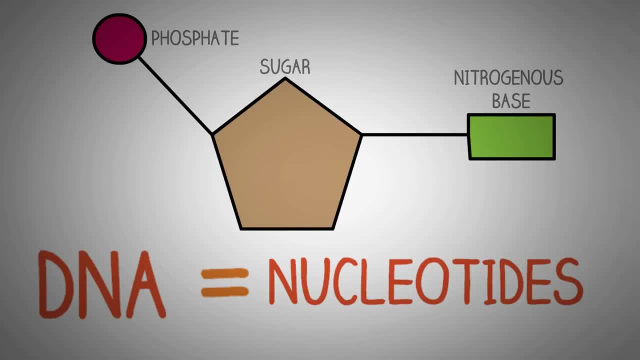 below and also on the top of the screen. But in a nutshell, you can conclude that the sugar present inside the nucleotide is called the deoxyribose, which is a 5-carbon sugar which belongs to the pentoses. The phosphate group consists of a phosphorus ion to which four oxygen atoms are attached, And then we 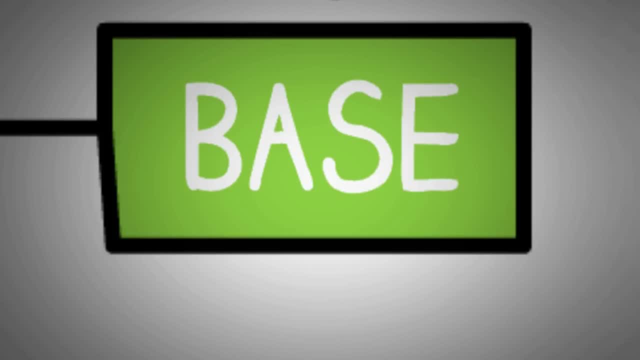 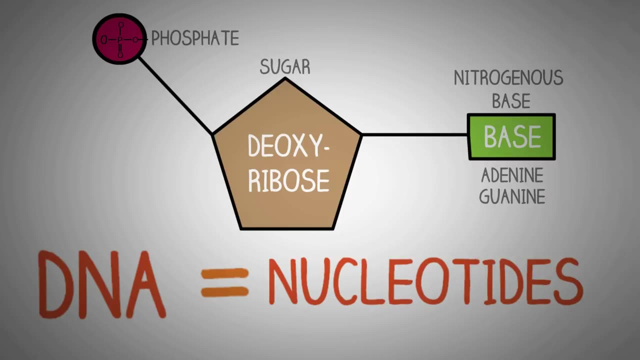 have the important nitrogenous bases, which are organic molecules which contain nitrogen in the form of ringed structures. We have four different types of bases that can be present inside the molecule DNA. So let's get started. So let's get started. 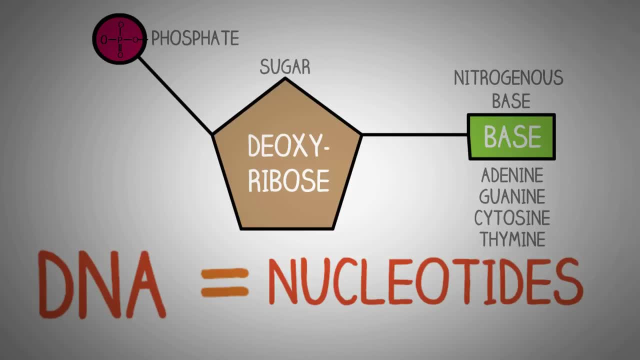 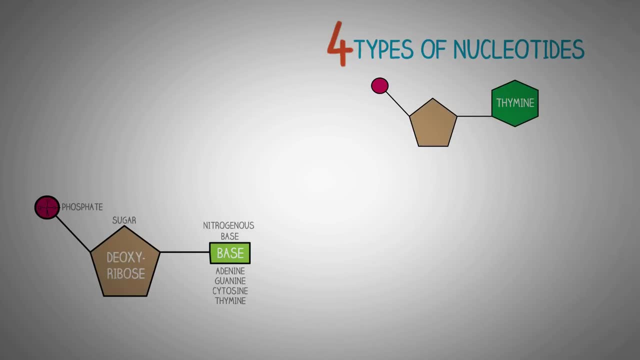 So let's get started Now. since we can have four different types of nitrogenous bases, we can have four different types of nucleotides that are present inside the structure of a DNA. Now, as you can see, these four nucleotides are arranged in two groups. The first group is known as pyrimidines. 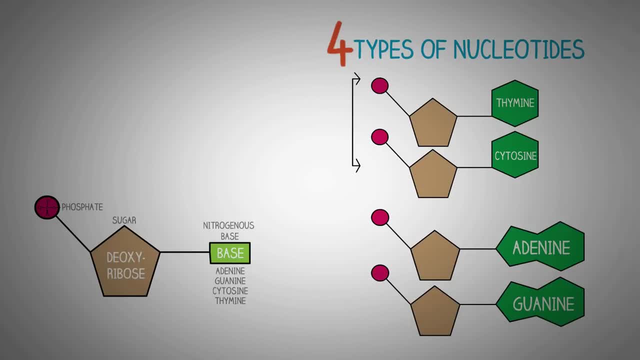 and these contain the nitrogenous base, thymine and cytosine, which are both single ringed bases, And the second group is called pyrimidine And the second group is called cytosine. And The second group contains the nucleotides, which are known as purines, which have adenine. 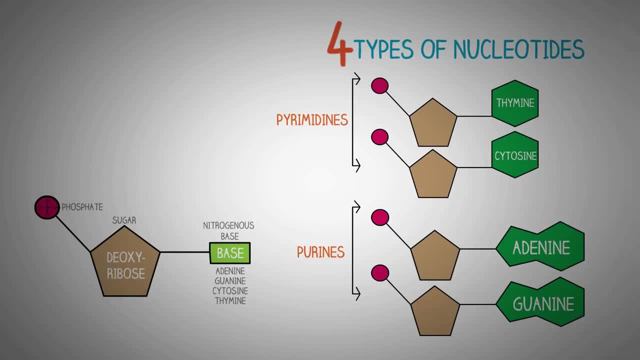 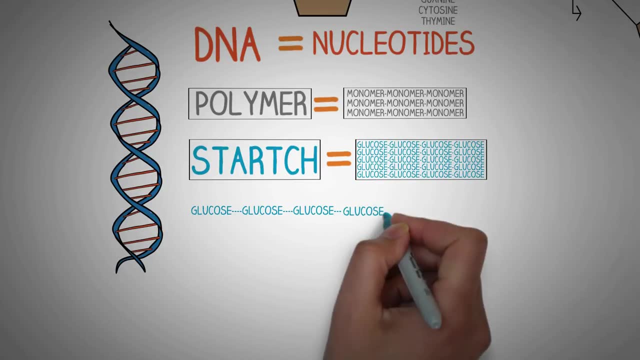 and guanine as the nitrogenous base, which are double-ringed structures. Now, in case of starch, the structure is pretty simple, which only consists of long linear chains of glucose, or either branched chains which are joined together by glycosidic bonds. 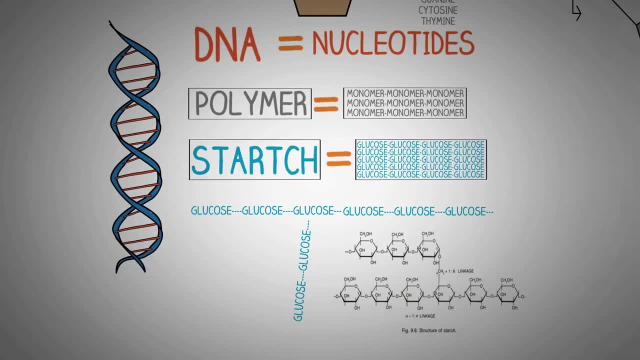 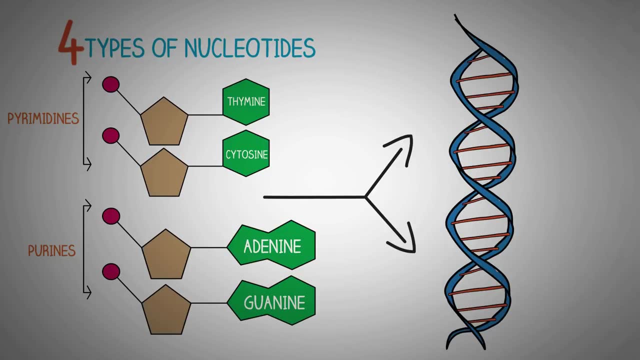 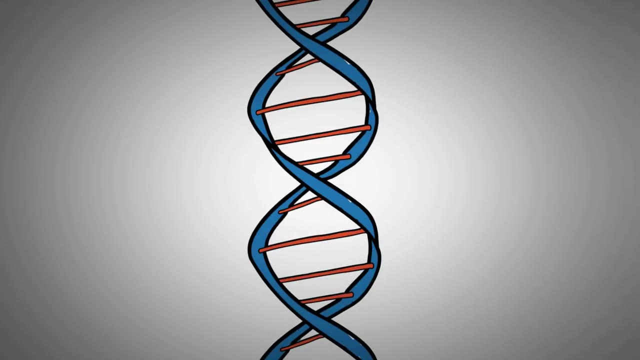 This is the chemical structure of the starch and you can see the different types of glucose chains. But in case of DNA, the four types of nucleotides join together in a very complex way to form the double helix structure. Now, if you zoom into the structure of this double helix model of the DNA, you can clearly 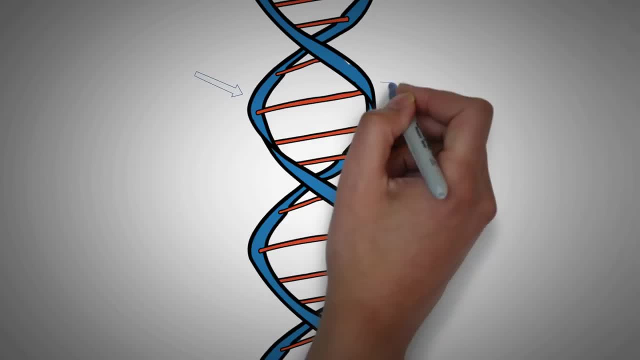 see that it basically consists of these two blue lines which are twisted around each other, and it also consists of these orange lines in the center which connects these two blue lines together. Now, to understand its structure in a better way, if we just untwist the double helical, 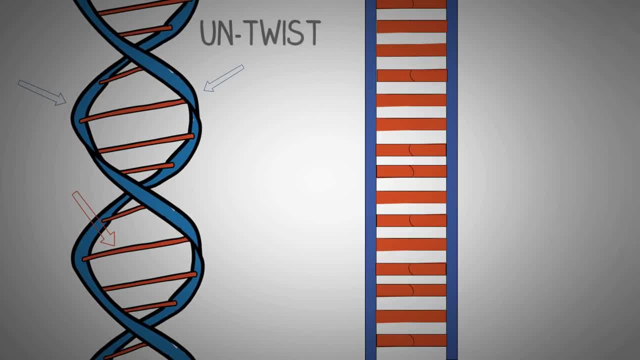 model, we will get something which is known as the stethoscope. This is the step ladder model of the DNA. It also has a similar structure and it consists of these blue vertical lines and these orange horizontal lines. Now, these blue vertical lines basically represent the sugar phosphate backbone of the DNA. 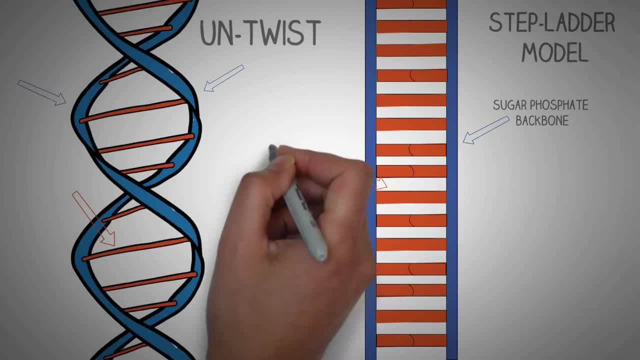 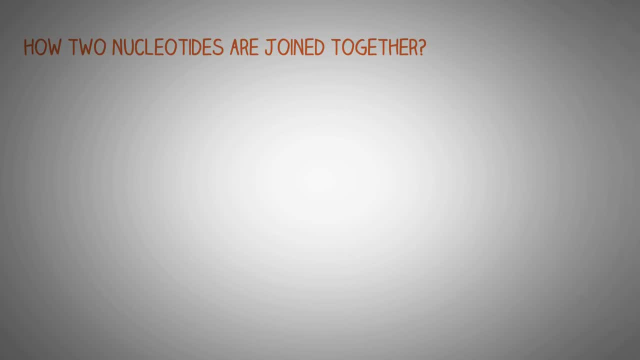 And the central lines, which are orange in color, represent the base pairs of the DNA. We will get to these terms in just a bit. Now, to understand this structure in more detail, the next thing we have to understand is how two nucleotides are joined together. 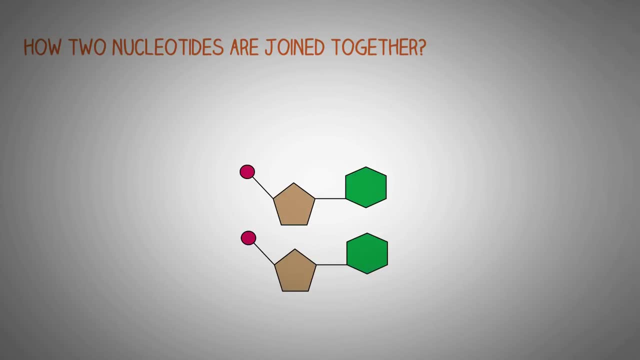 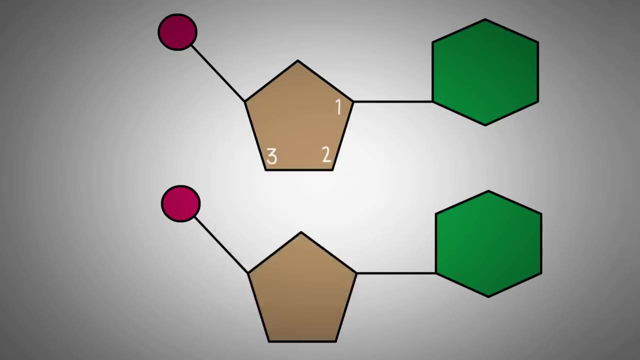 Basically, we covered this topic in our previous video, So if you want to learn in more detail, you can refer to that video. The link to that video will be in the description below. Now the carbons present inside the deoxyribose sugar of the DNA are numbered from 1 to 5. 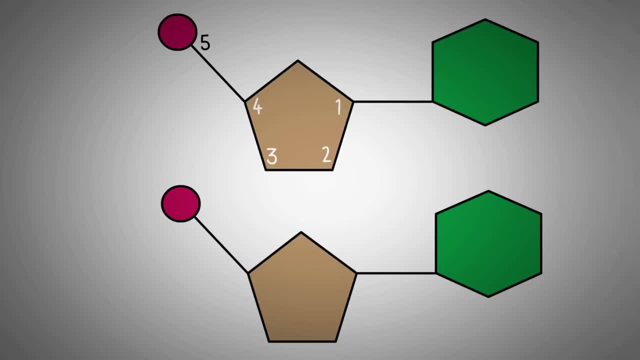 in the clockwise direction, And you should remember this numbering of the carbon atoms because it will help you to understand the concept of directionality of DNA. Now what happens is that the third carbon in every deoxyribose sugar forms a bond with the phosphate group of another nucleotide that is present below it. 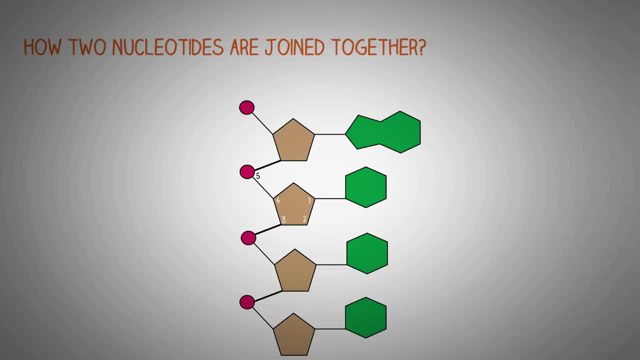 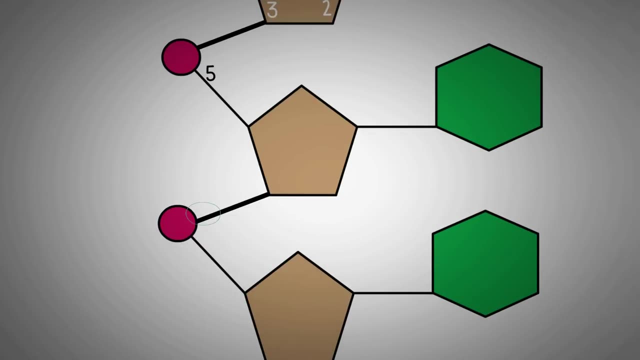 And this bonding extends in both directions. Now, if we zoom into this structure, you can basically see that every phosphate is connected to two sugars: One bond with the third carbon of the sugar above and one bond with the fifth carbon of the sugar below. 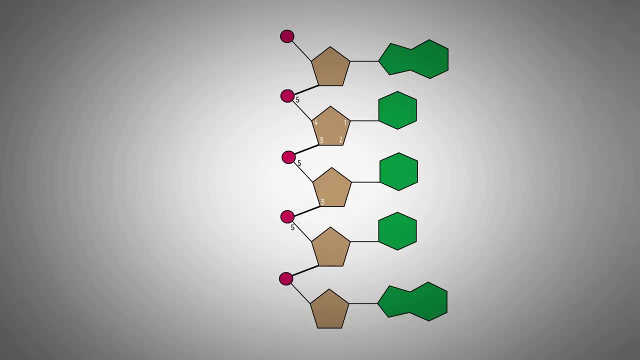 And now again, if we zoom out, you can clearly see that, due to the bond formation between the sugar and phosphates, we create this sort of sugar phosphate backbone on one side and we have all the nitrogen. So what this basically represents is essentially a single strand of DNA. 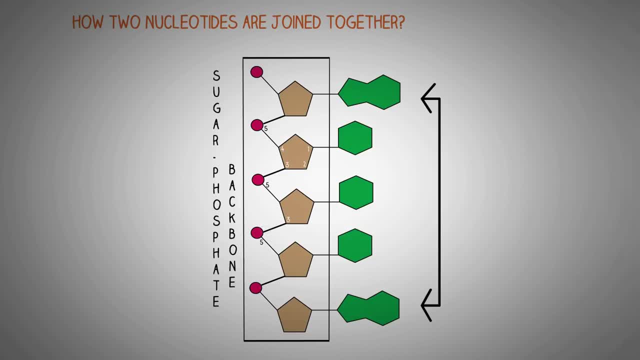 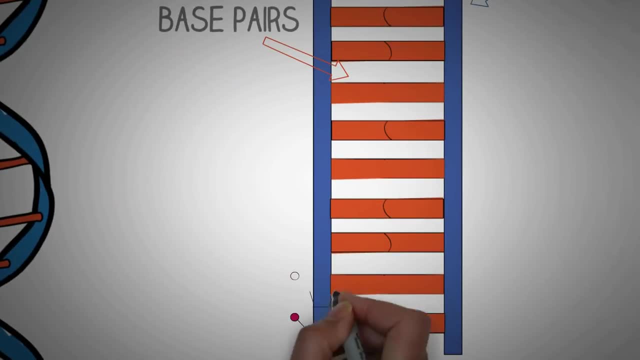 Now, if you go back to the stepladder model of the DNA, you can clearly understand how the different nucleotides in a single strand of DNA are joined together to form the sugar phosphate backbone, which was represented by these blue vertical lines And in the center we had these orange bars which connected these two lines, which are 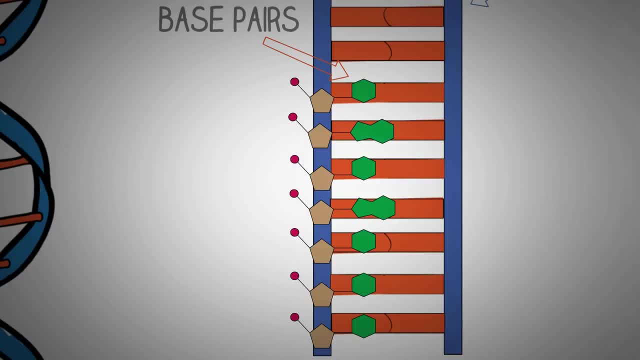 essentially the base pairs from one side. Now, if we zoom out, you can clearly see that the base pairs are connected to each other. Now in the opposite side, we have the other strand of the DNA, which is quite similar to this original strand but has some key, important differences for you to understand. 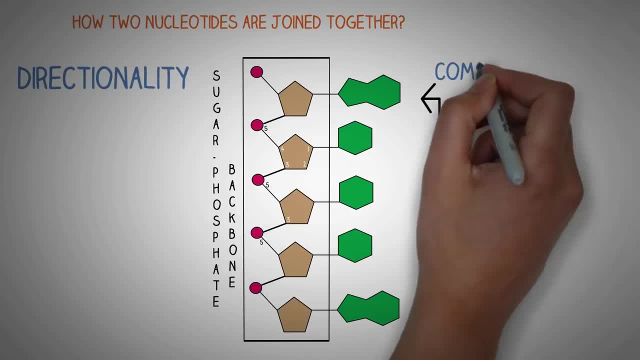 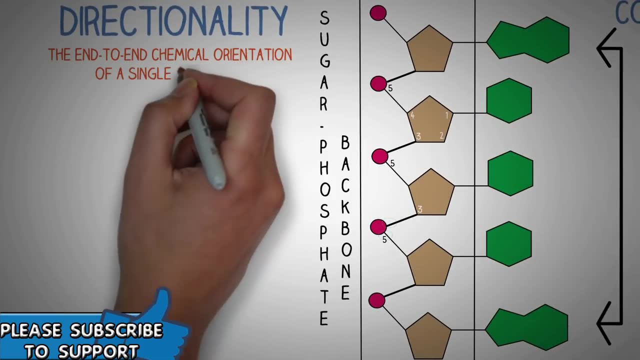 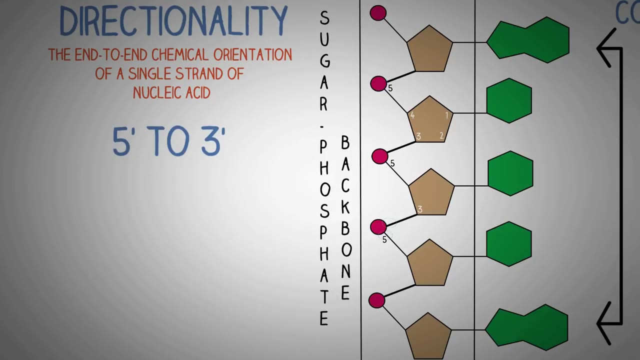 And to understand these key differences, you have to understand the concept of directionality and complementary base pairing. Now, what directionality essentially means is that it is the end-to-end chemical orientation of a single strand of nucleic acid. In this example, you are seeing the single strand of a nucleic acid. 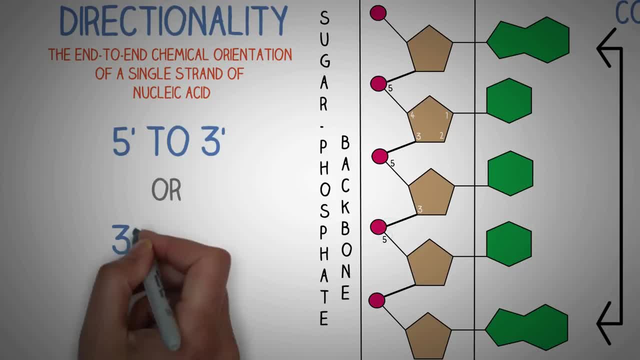 Now the direction of the DNA is expressed by the nucleotides. Now the direction of the DNA is expressed by the nucleotides. Now the direction of the DNA is expressed by the nucleotides. However, they are� Spaß 1979-18.. 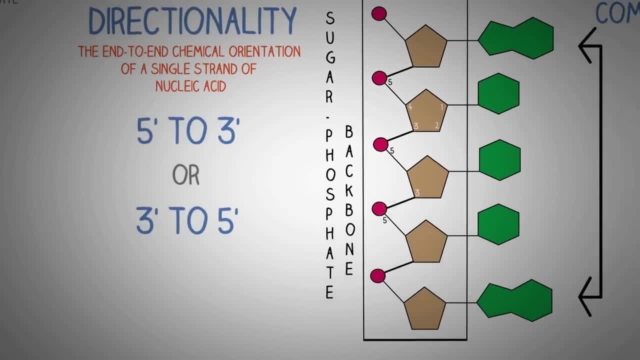 Now the DNA can be expressed in 2 ways: 5' end to 3' end or 3' end to 5 end. Now, if you look closely at this structure, you can basically see that it currently has a 5' end to which a phosphate group is attached. 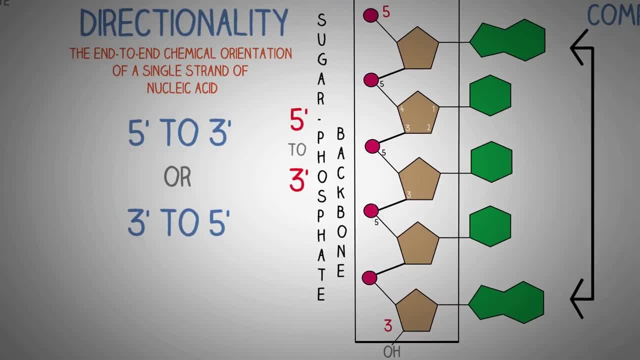 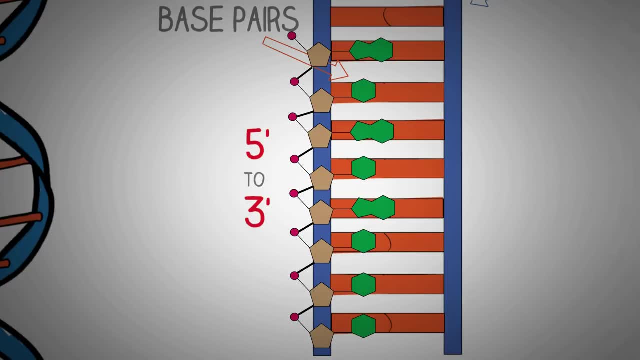 And it also has a 3' end below to which a hydroxyl group is attached. So if you come back to our DNA liler model, we can see that the strand we made before runs in the 5'-3' direction. 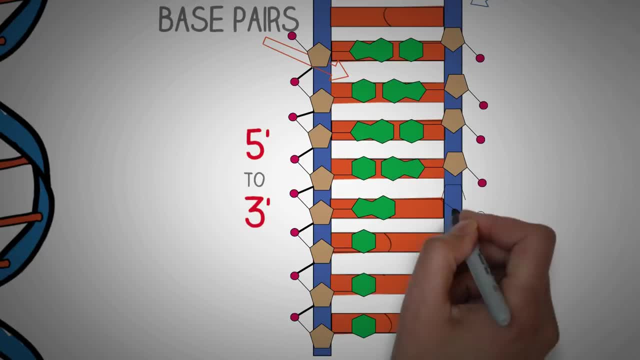 at the opposite strand. you can basically note that there is one important key difference: that it runs in completely opposite direction. It has its 3' end in this direction and its 5' end in this direction, So it is said to be running from 3' to 5' direction, which 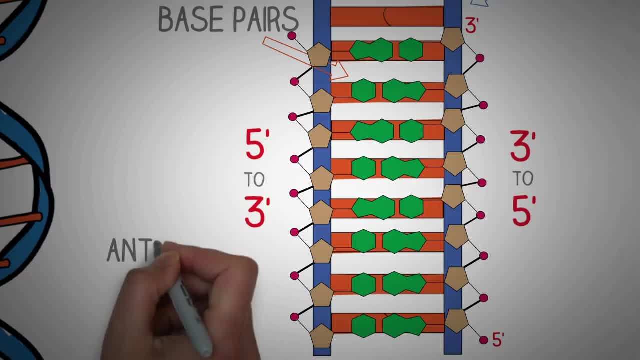 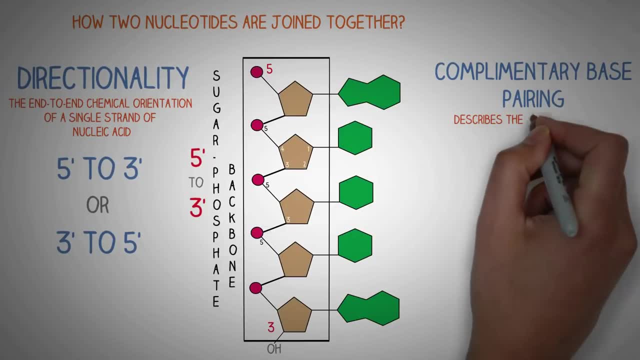 makes the two strands of the DNA antiparallel. Now the next important thing for you to understand is the complementary base pairing, which describes the manner in which the two nitrogenous bases of DNA strands align with each other. So it basically means the base adenosine always. 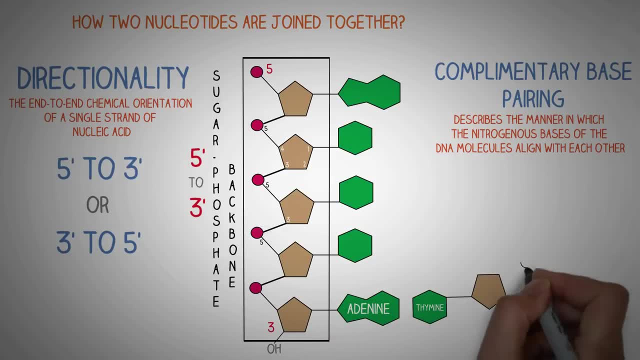 pairs with base thymine and base guanine always forms Hydrogen bonds with Basetocene. You can see this rule in action in the DNA stepladder model, where you can see that base A always pairs with base D and base B. Now, with the DNA stepladder model still ausán, the other número is: we are makingur, but the base A always pairs with base T, so it will continue to stay the same. So we can então parece that the base A will always pair with base D and base B. If we take a bit more of our knot, we can see that. we can see that both are A and A goes side to side, So we can expect. 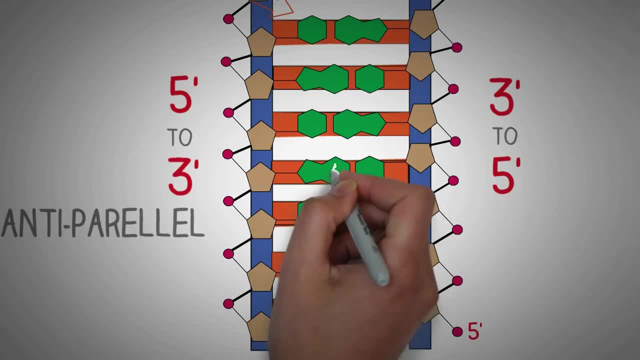 base c always pairs with the base g. these bases are essentially forming the hydrogen bonds in the center which holds these two strands of the dna together. now the complementary base pairing is very important in one of the most important aspects: that it maintains a proper distance between the two strands of the dna, which is very, very important for the stability of the two strands.